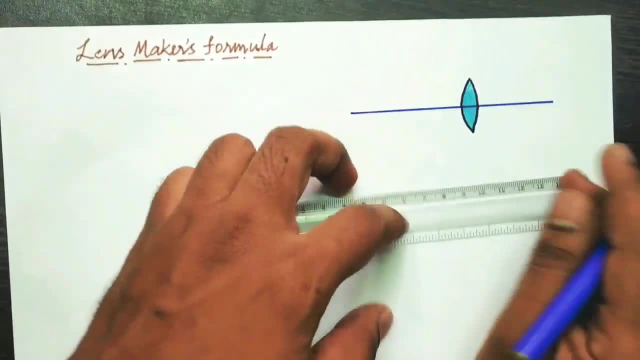 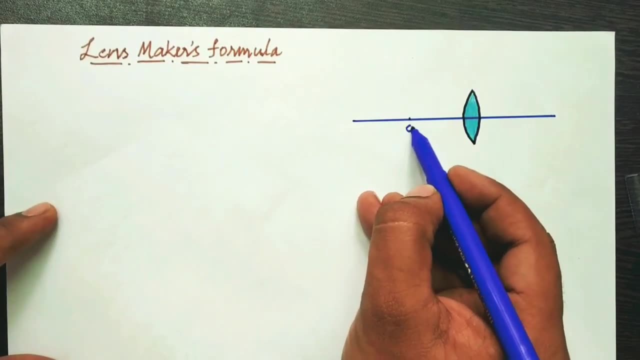 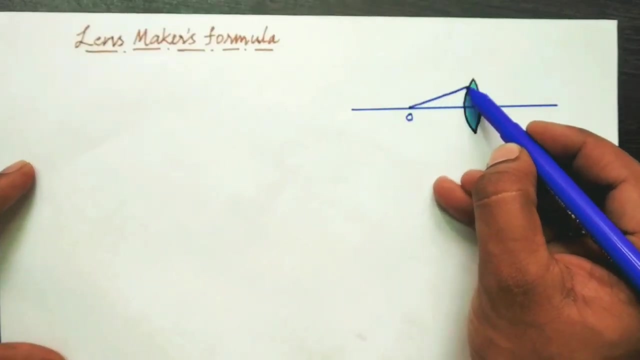 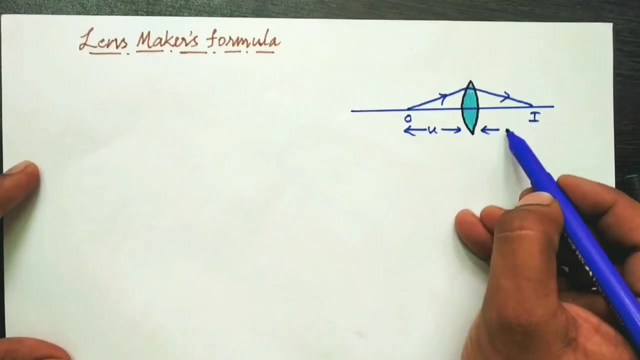 optical center of the lens. such a way it also passes through the centers of curvatures of the two surfaces. Now let us say this is a point object. we assumed already it has to be done with the point object O. So now let us say this is an incident: ray falls on the first curved surface, refracts into the medium and finally comes out. The image forms at a position i. Let me take this as object: distance u and image is formed at a distance v. 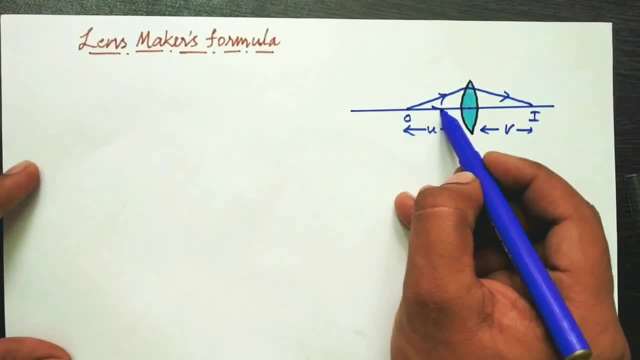 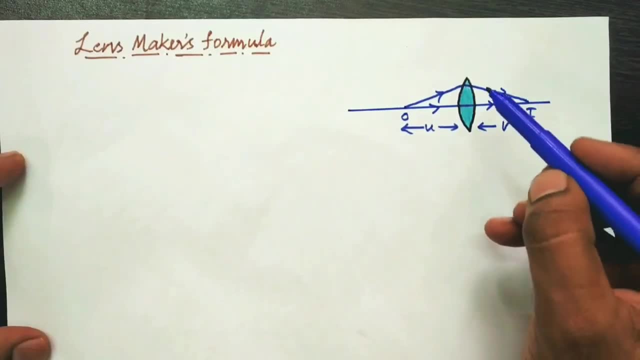 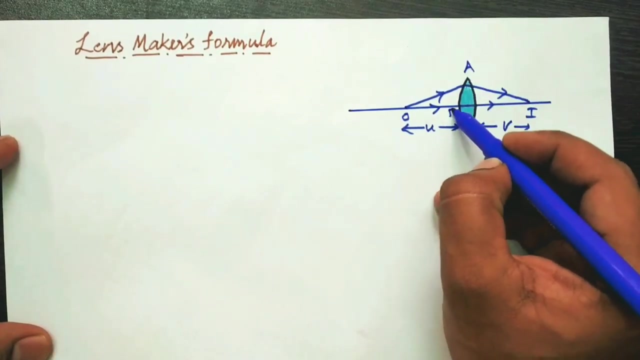 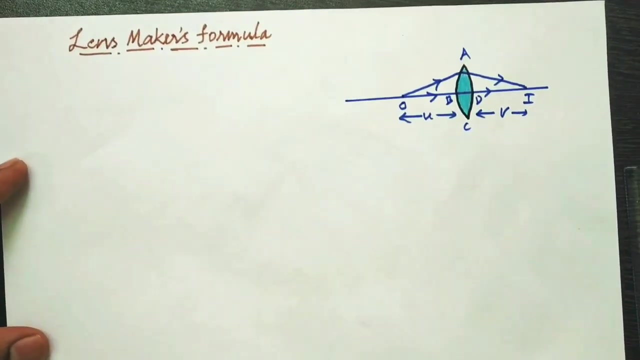 And we also consider one more light ray that passes through optical center. It doesn't deviate. So that is the point where image is formed. finally, Right, So the image formed by the convex lens is due to the two curved surfaces. Now what we are going to do? let us name this curved surface as ABC and ADC. There are two curved surfaces Now. first curved surface, we will take now that is ABC. 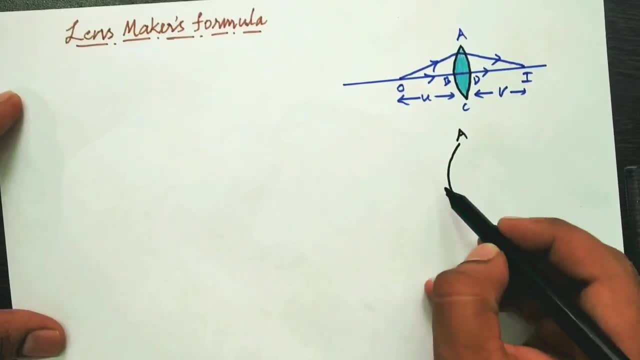 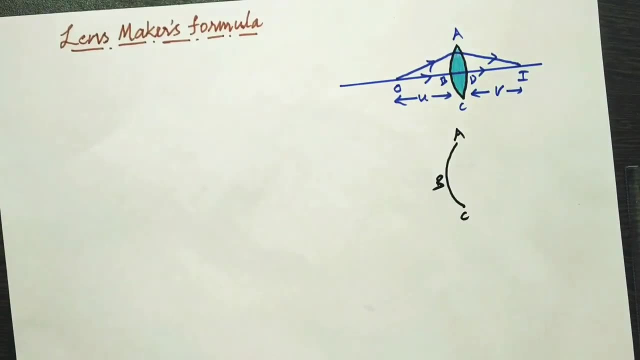 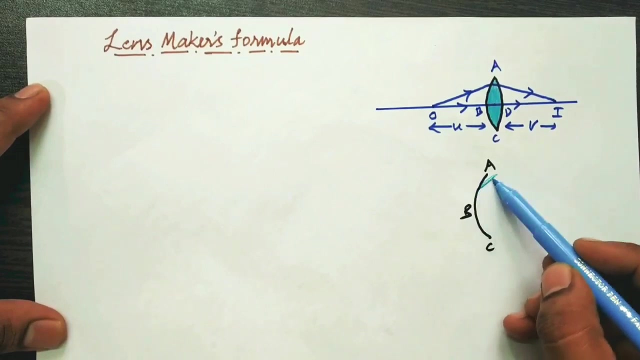 So first curved surface, ABC, the image formed due to first curved surface. we first find out and then that image acts as object for the second curved surface. Finally, the image forms at v. Let us see how it goes Now for the first curved surface. the second part is denser medium. 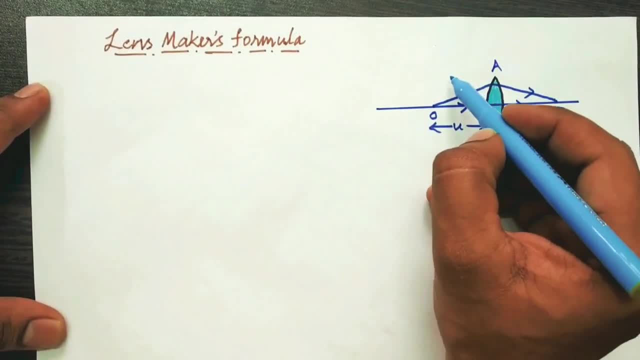 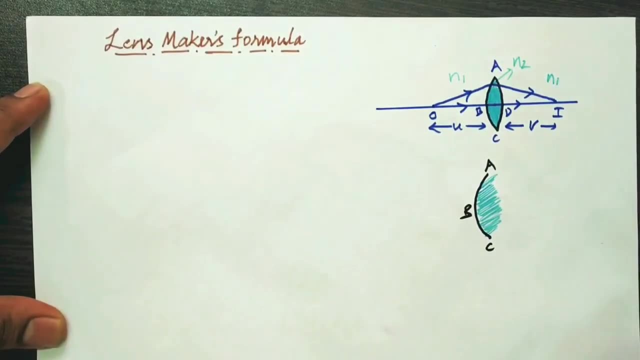 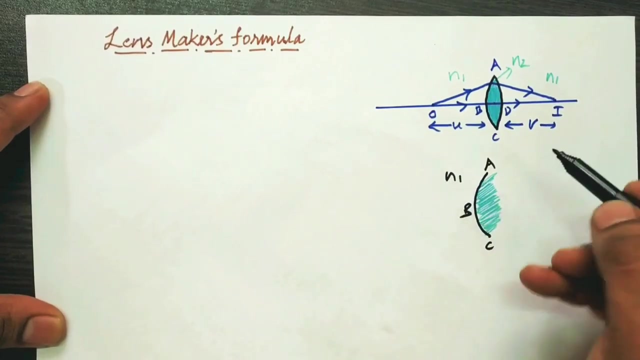 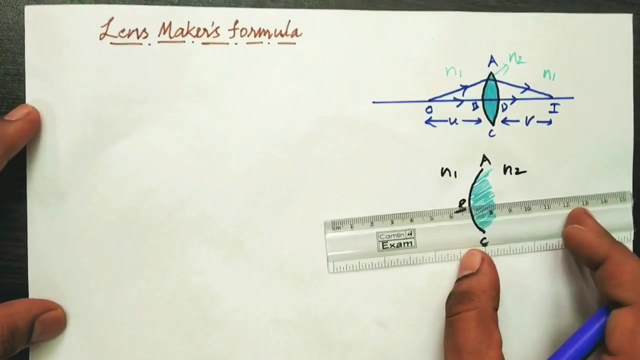 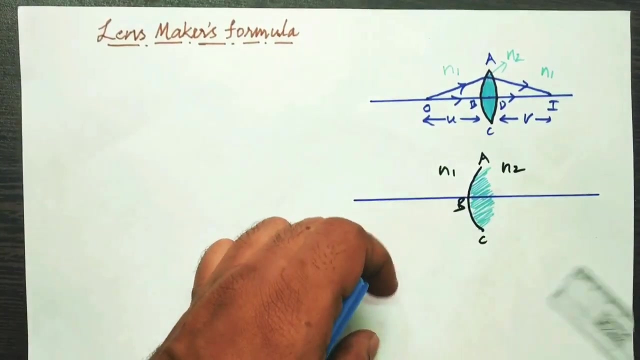 Now let me name these radar medium and denser medium. First, N1, that is surrounding medium. N2 is the surrounding medium. N3 is the surrounding medium. N4 is the surrounding medium. N5 is the surrounding medium. This is the medium of the lens. back to N1. So here I am considering only one curved surface. So this is the radar medium. N1. This is denser medium. N2, because I am considering only one curved surface. Right Now let me draw the principal axis for this spherical surface. So in the same way, the one which is drawn from the pole of the spherical surface. 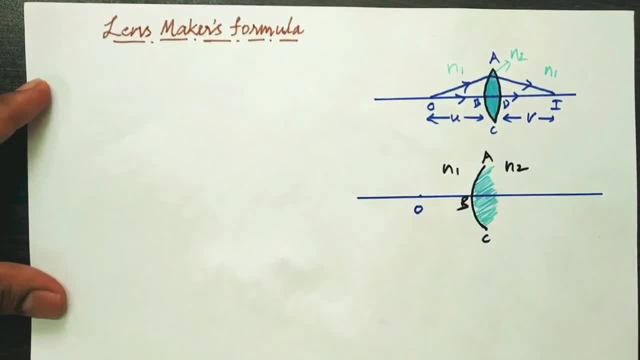 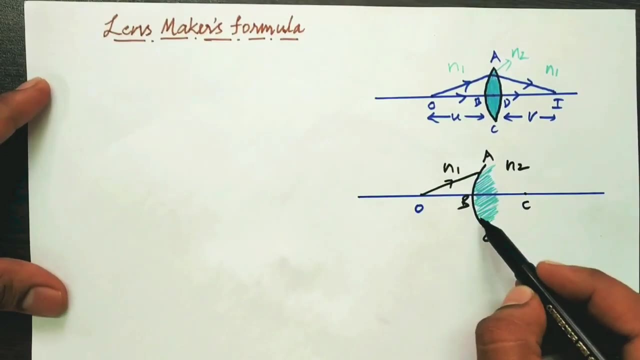 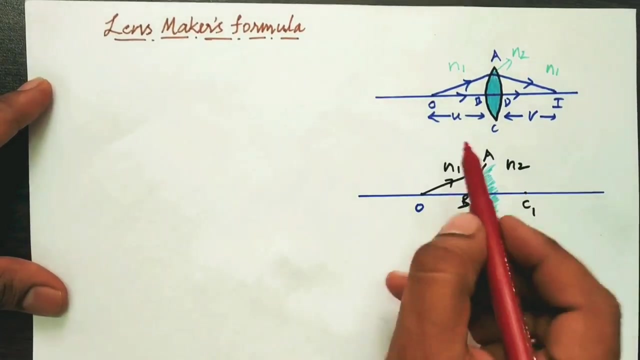 Now let us take the same object, O point sized object. Let us draw incident ray at the first surface now. Now the second step is drawing center of curvature. This is the center of curvature of this piece. So let us name this as first surface of C1.. Now let us draw the normal at this point of 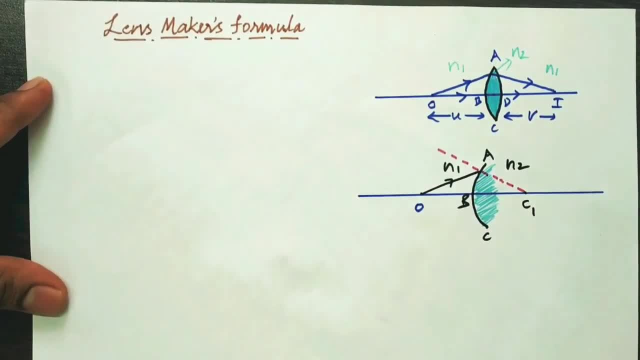 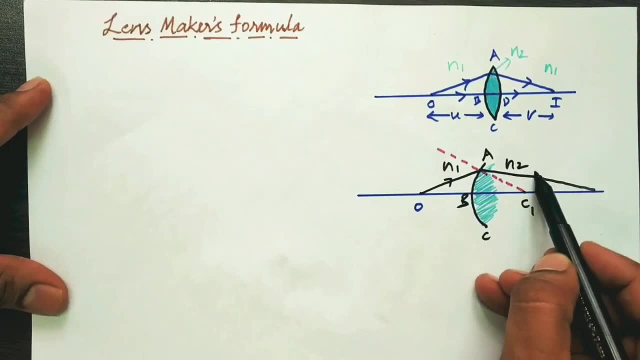 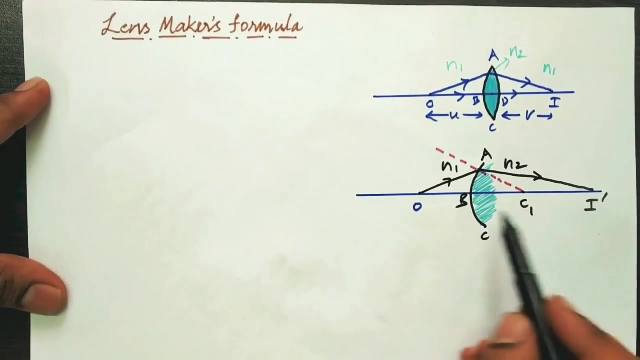 incidence. So what is normal? The line drawn from the center of curvature to the point of incidence. Now, light ray traveling from rarer to denser, it travels close to the normal. So here, image is formed due to the first surface. let me name it as I dash: This image is formed. 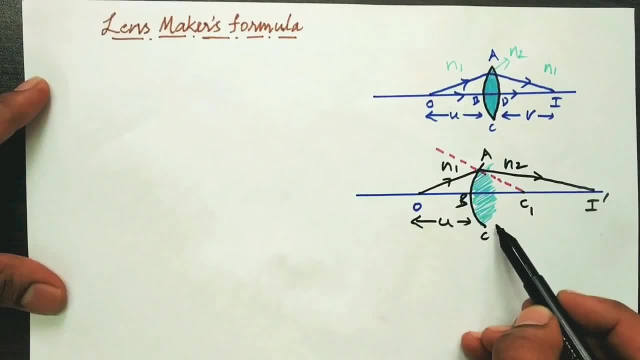 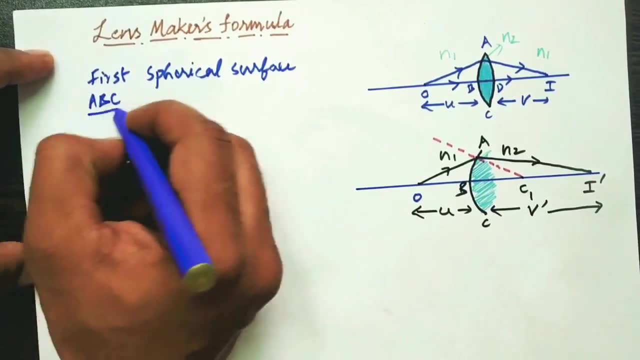 due to ABC. This is object distance U and let me take this as image distance V dash. Now from the first spherical surface ABC we apply an important relation, that is, refractionate spherical surface N2 by V-1.. Now, from the first spherical surface ABC we apply an important relation, that is, refractionate spherical surface N2 by V-1. 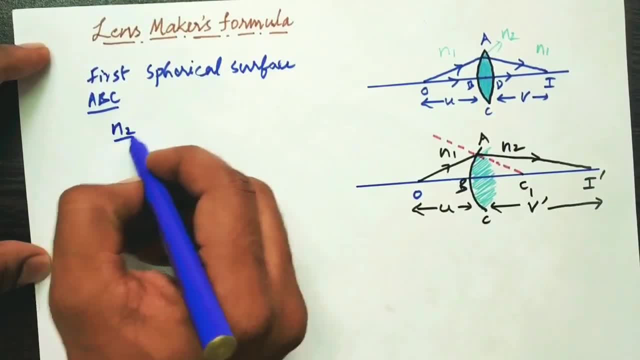 Now from the first spherical surface, ABC, we apply an important relation that is refractionate. the second Kanel directionاه expression is equal to: about n1 by U is equal to N2 minus N1 by r, N2 by V-1.. 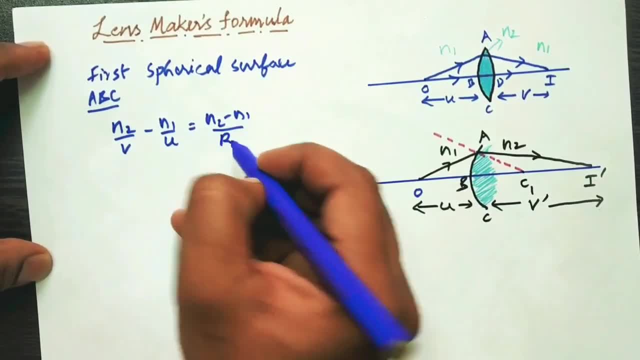 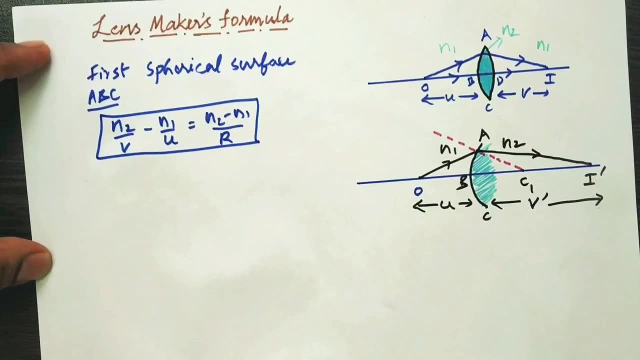 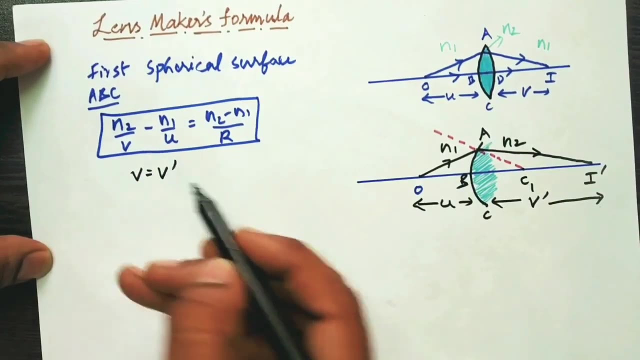 This is the version that is been uploaded in my channel. Y ou may goa through the derivation of easy to understand the topic. Now let us substitute the values N2 by N1. will remain unchanged- for n values v-dot. This is the image which is formed due to the first surface. R is r1.. 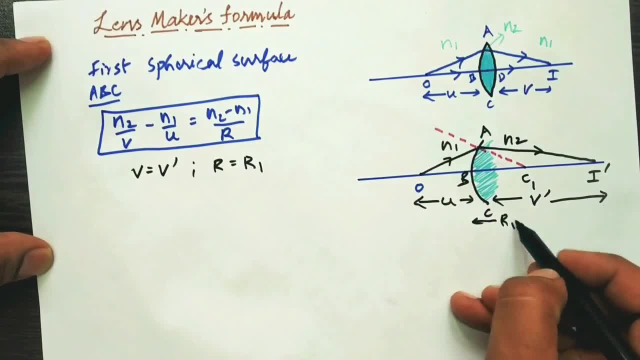 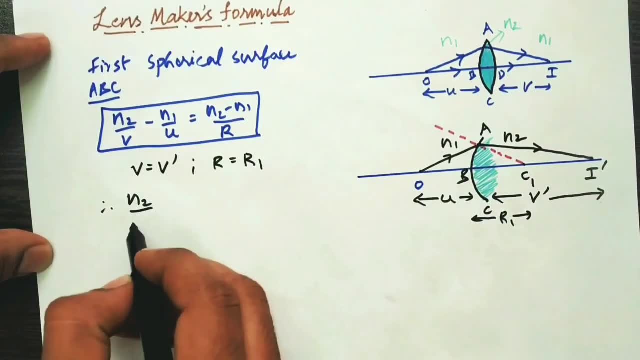 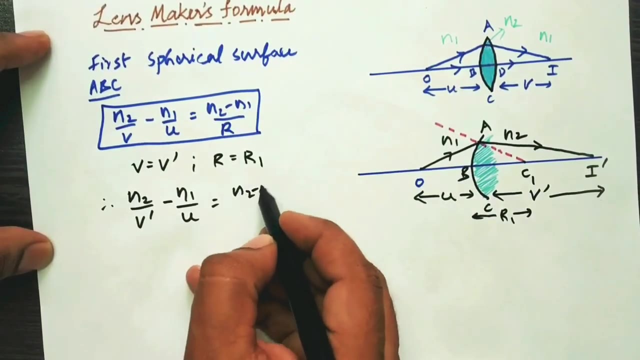 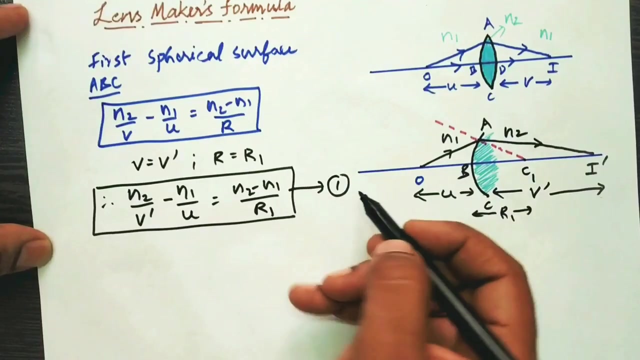 let me name this as r1, that is distance between pole to the center of curvature of the first surface. now the relation becomes n2 by v. dash minus n1 by u is equal to n2 minus n1 by r1. this is first relation. now let us take this as equation number one. 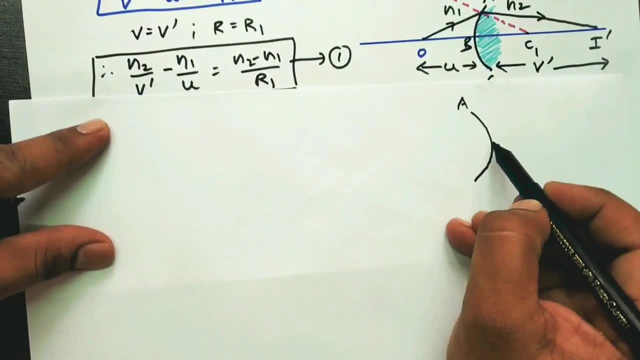 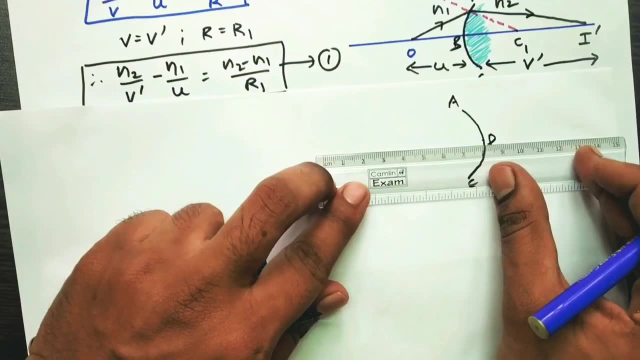 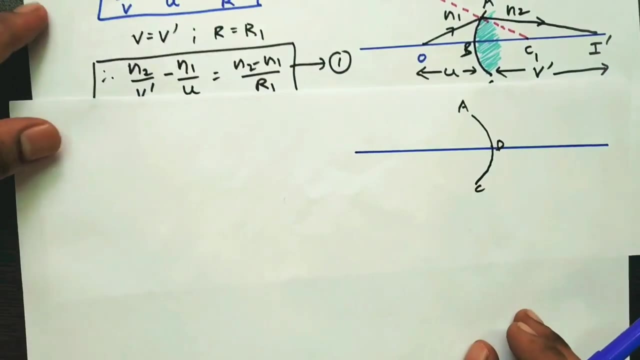 now let us apply the same formula for second spherical surface, Adc. so on the whole, the final image is formed due to both of the spherical surfaces. so let me draw a principal axis for the second surface, that is, adc. now here the image formed due to the first spherical surface. 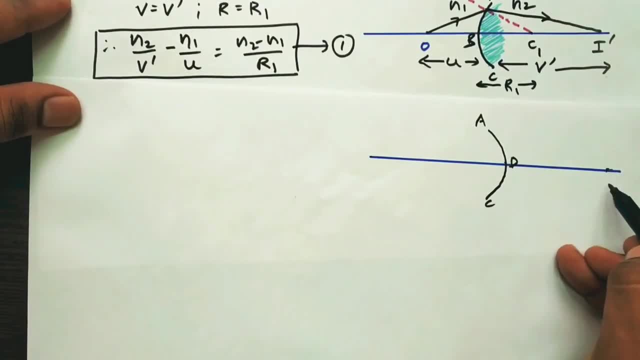 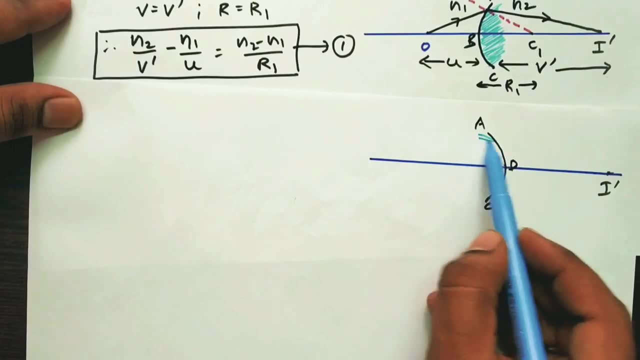 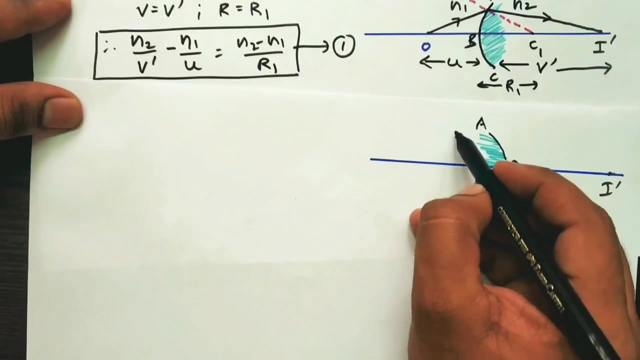 acts as the object for the second spherical surface. so here i dash: acts as object. so now this is the spherical surface in which the light ray now travels from denser medium to rarer medium. So earlier, rarer to denser. now light ray is coming from denser to rarer. 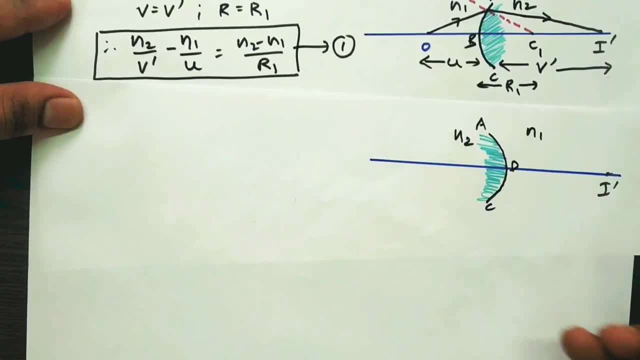 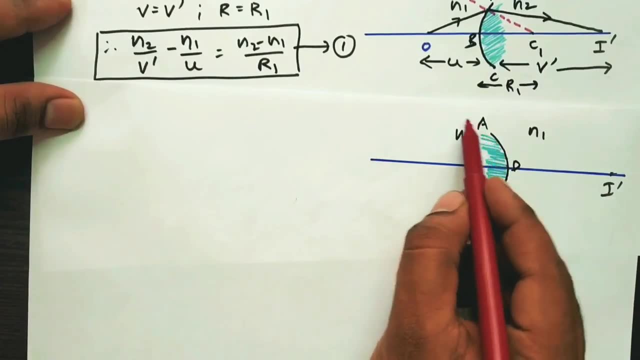 So N1 here, N2 and N1 gets reversed. This is very, very important change that we need to notice. Now let us draw the normal to this. This is the center of curvature of this spherical surface. Now this, the line that, drawn from the center of curvature C2 becomes the normal at the 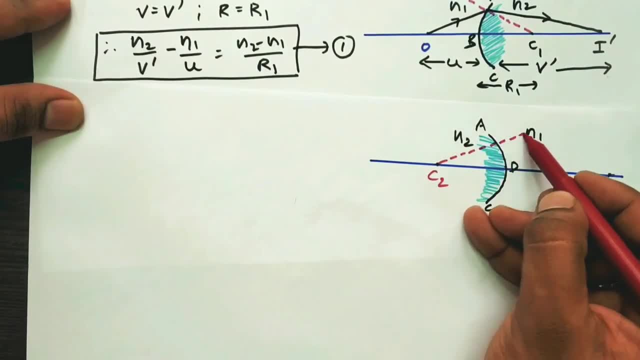 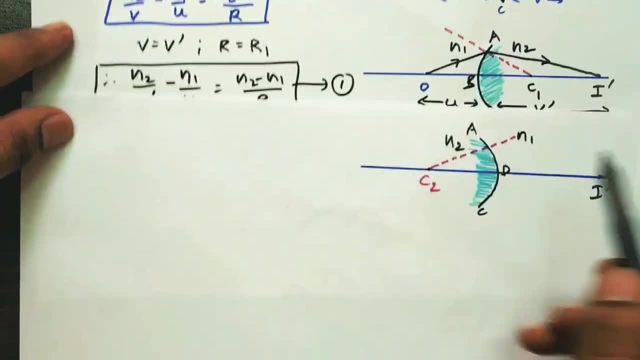 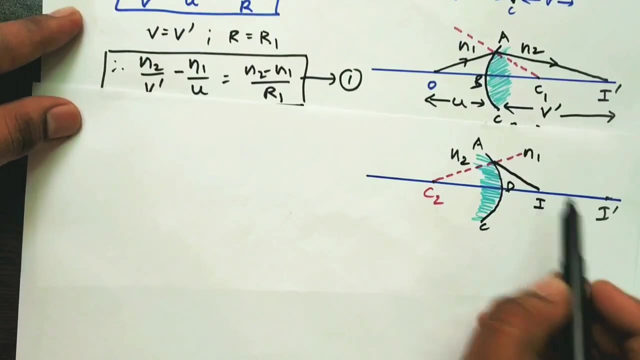 point of incidence. Let me draw the normal here. So the final image is formed here as the light ray traveling from denser to rarer medium, the light bend away from the normal. So here the final refracted ray comes like this, which is away from the normal and the 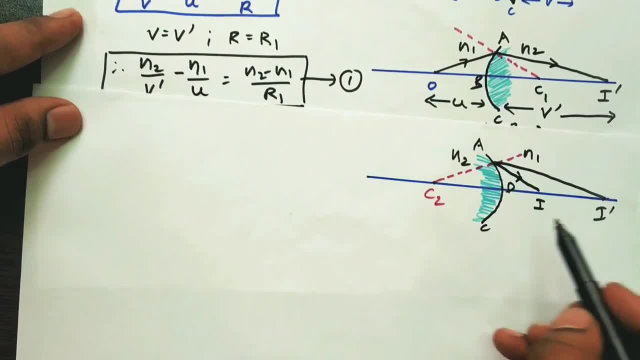 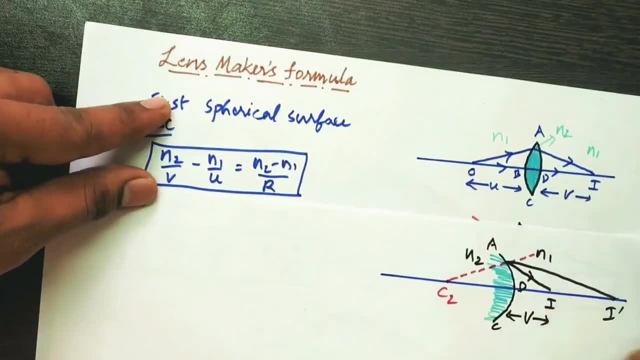 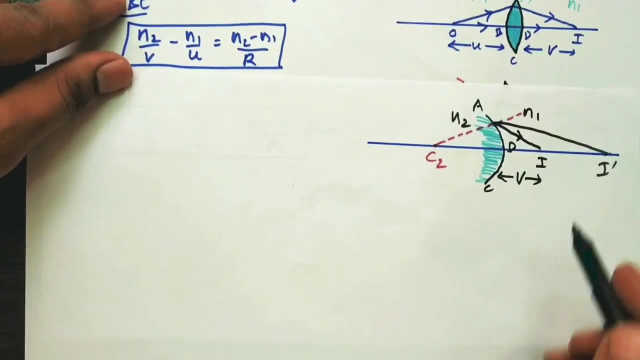 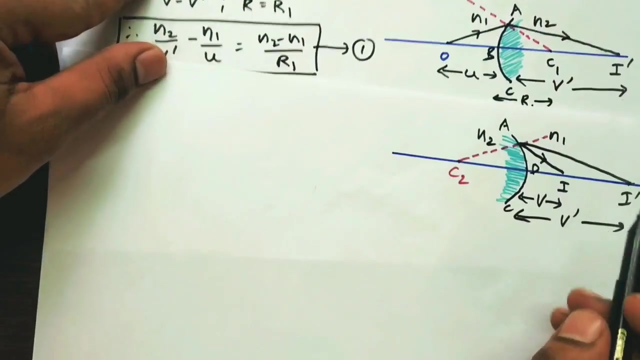 image is formed at here. This is the object distance. Virtual object. Generally we do not see the virtual object. This is actually the final image formed by the lens. So V is the final image distance formed by both of the spherical surfaces. Now, if I apply this distance, we all know it is object distance. for the second surface. 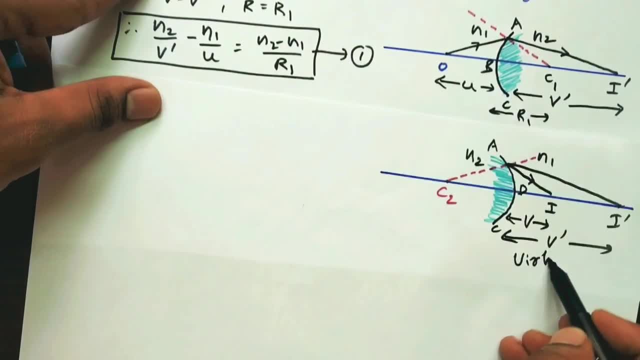 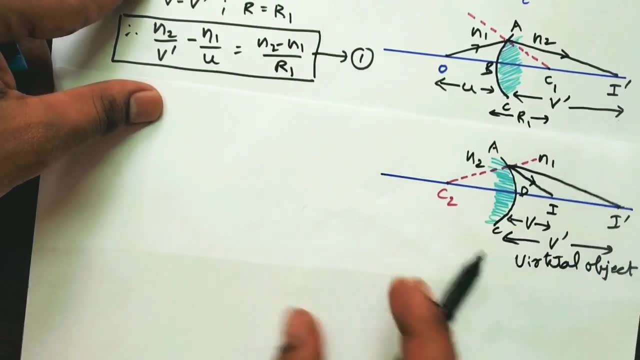 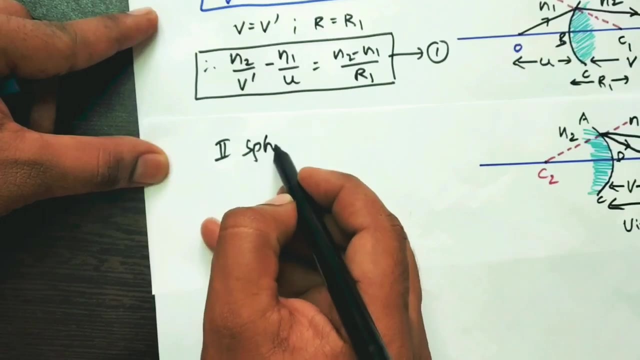 So V' is object distance for the second surface. So we call this as actually virtual object for the second surface. We cannot see the virtual object. Now let us apply the same relation for this. Now, the important change that you can see for the second spherical surface is: 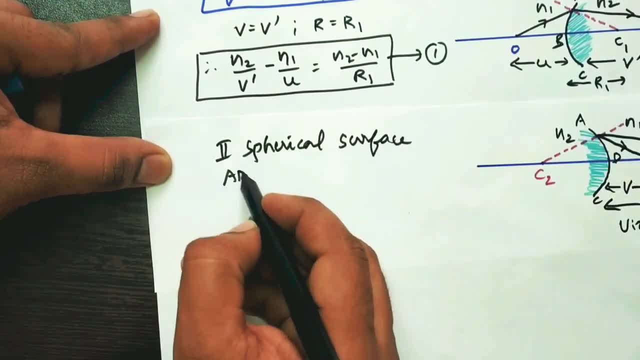 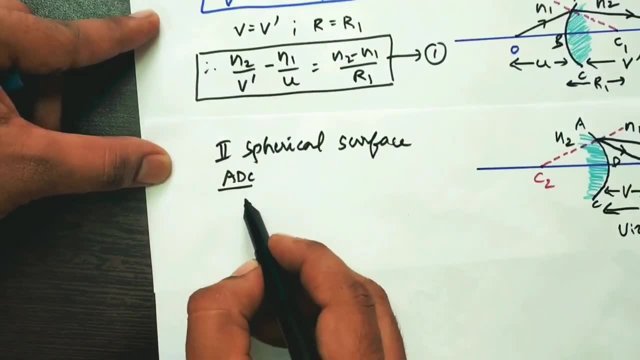 Now N1, N2 places get interchanged. Now let us apply for the second surface, ADC. If you see, there N1, N2 got interchanged. So in the place of N2 I am writing N1. now N1 by final image is V minus N2 by object distance. 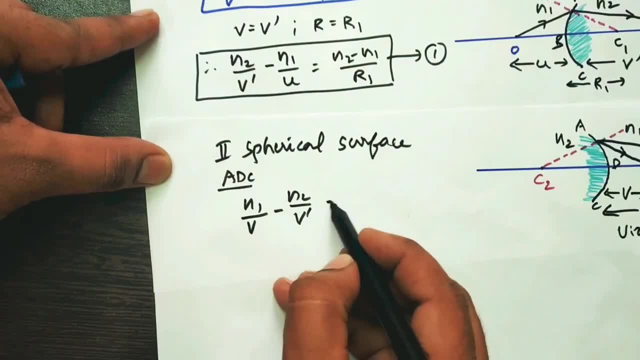 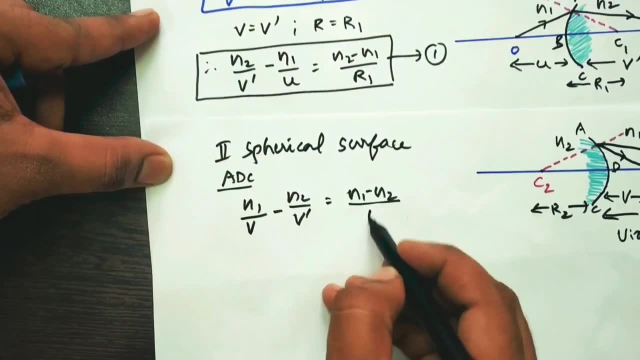 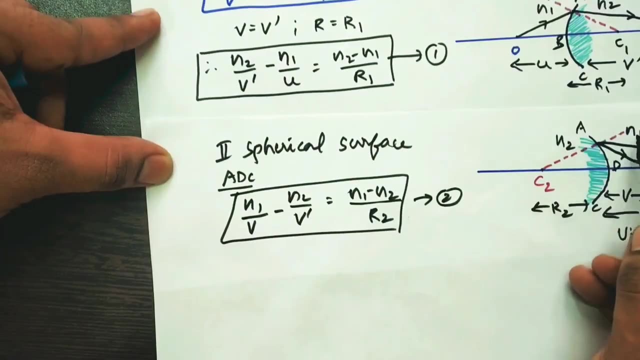 I told you already, V' acts as object distance, So V' is object distance is equal to N1 minus N2 by the second radius of curvature, So R2.. This is very important, Alright, So here the change is N1, N2 got interchanged. 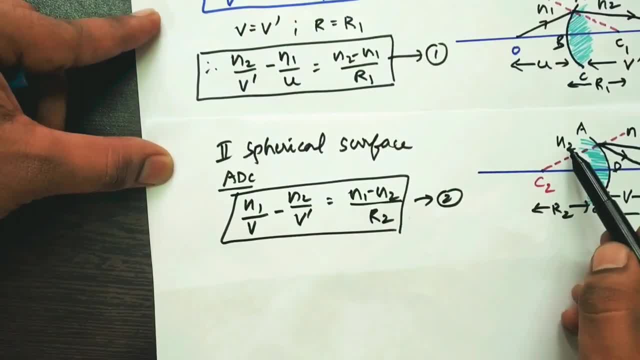 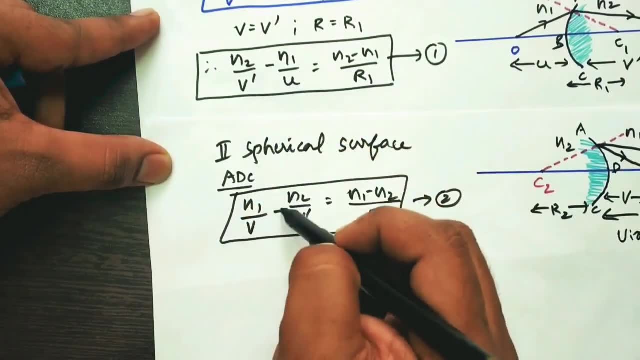 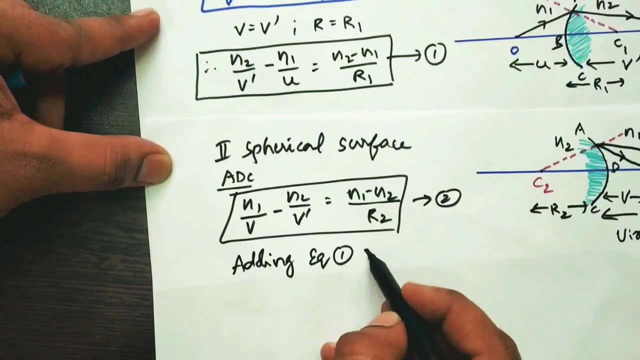 In the place of U. we took V' in the place of V, as it is V, we took right. So if you understand this, it is very easy. Now, if we compare these two equations, it is very clear: by adding those equations, we can neglect that virtual object thing. 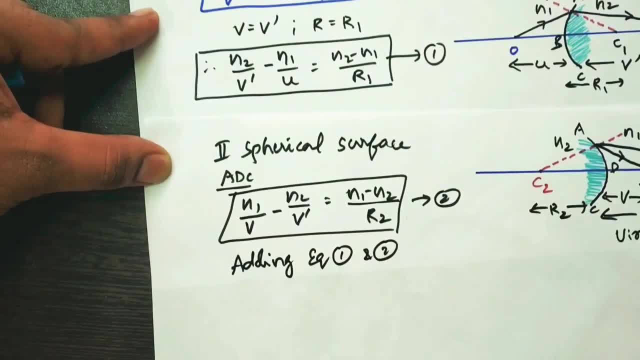 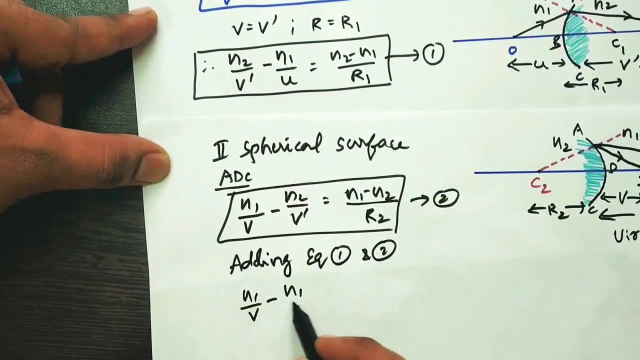 That means V' we can neglect. See here: this is in the equation one. if you observe, this is N2 by V' plus, this is N2 by V' minus. It gets cancelled. Cancel the V' terms. and if we write the remaining equation, it becomes N1 by V minus N1 by U is. 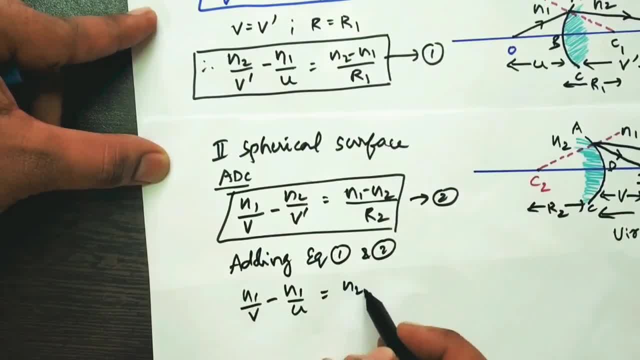 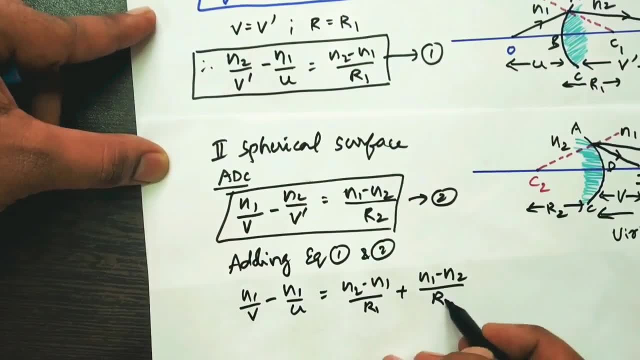 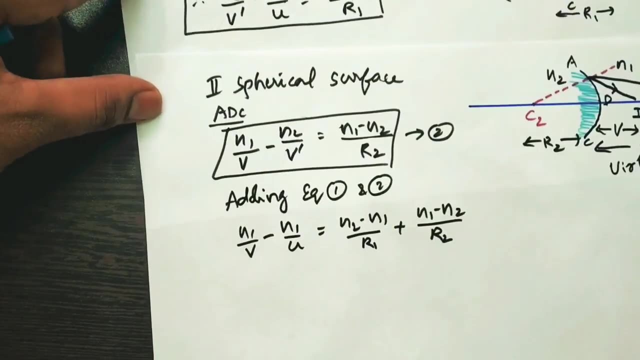 equal to RH, as I am adding N2 minus N1 by R1, plus N1 minus N2 by R2.. Here one more change. you need to notice Right: N2 minus N1.. N1 minus N2.. Now what can be taken common? 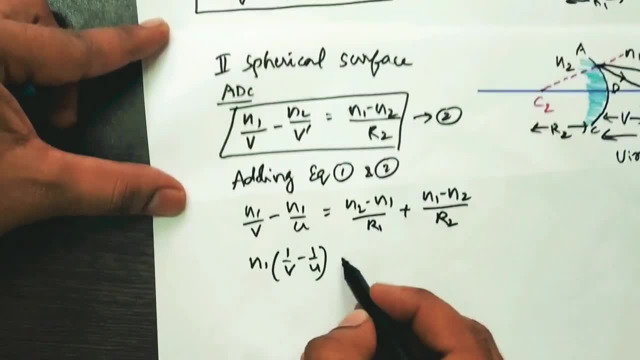 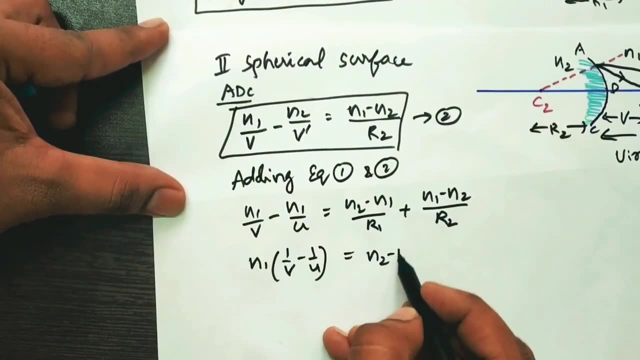 Here N1, 1 by V minus 1 by U. Now, very important thing here: N2 minus N1, I am taking it common. If I take N2 minus N1, common as the first is same but second is in reverse. so I will. 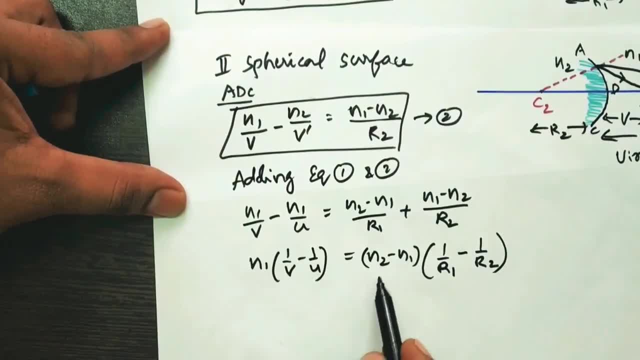 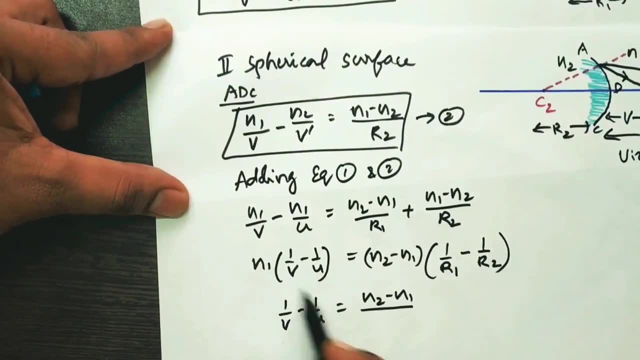 get minus symbol over there Right. So now N1. I am transposing to right hand side N2 minus N1 by N1.. Into: 1 by R1 minus R2.. 1 by R1 minus 1 by R2.. 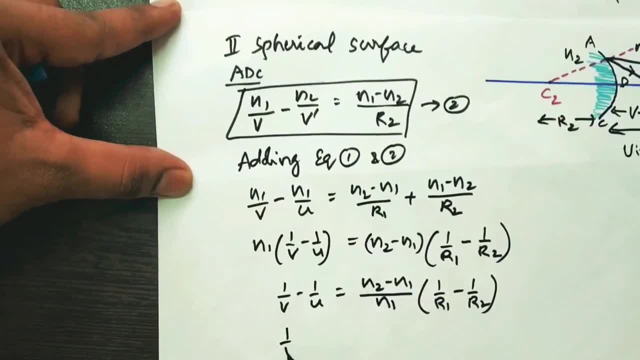 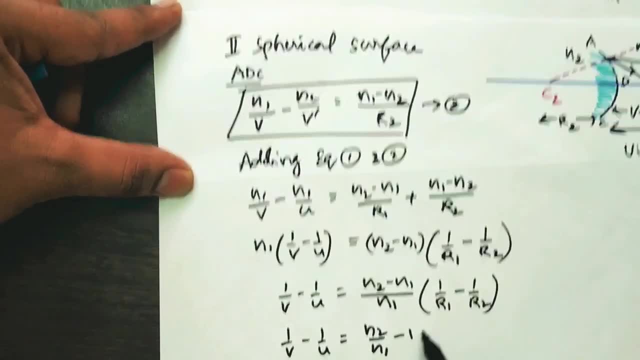 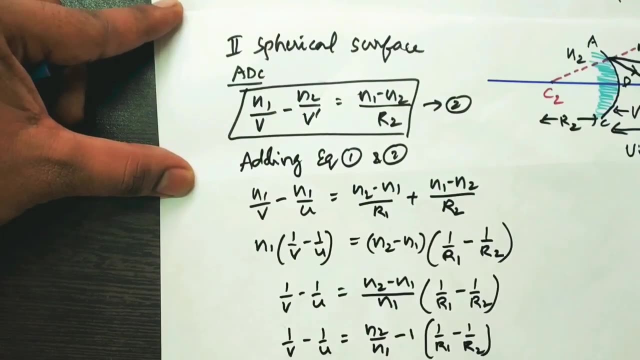 Right Now, 1 by V minus 1 by U equals to N2 by N1 minus N1 by N1 is equal to 1.. 1 by R1 minus 1 by R2.. Now, this is an important part. From now, what do we do? 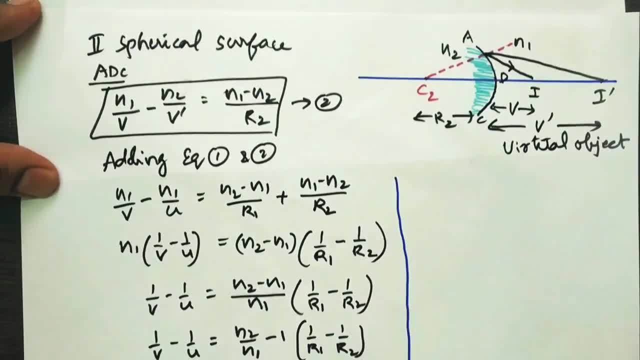 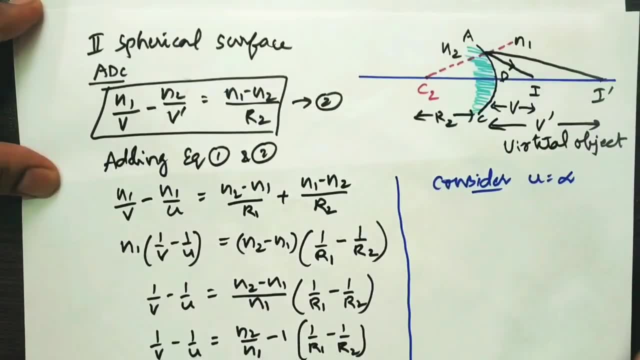 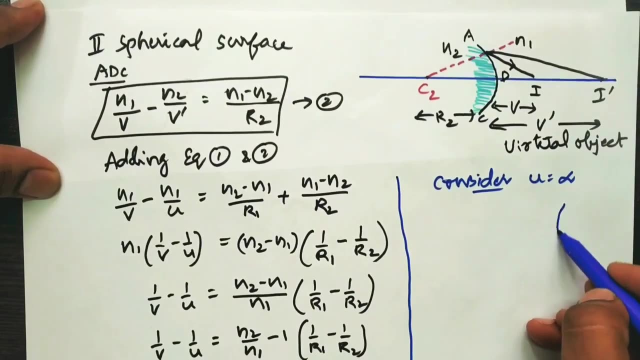 We consider the object is placed at infinity. Right Now, consider object is placed at infinity. where does the image formed by the convex lens? So, if we talk about the convex lens in which light rays are coming from infinity, So we know light rays coming from infinity converges to focus, isn't it? 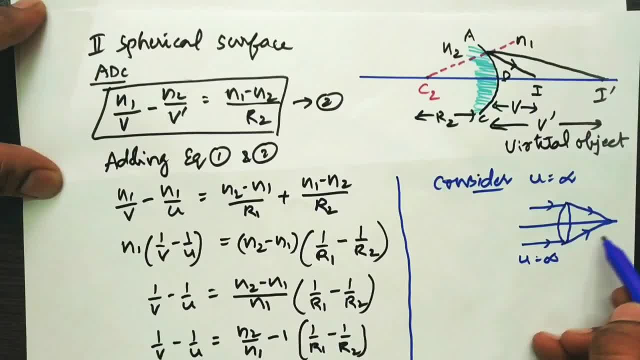 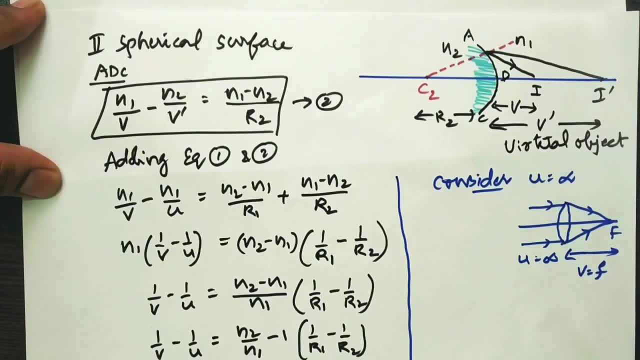 So there the image is formed, So object infinity. image is formed at focus. So V is equal to F Right, So image distance is F Right. So if I substitute those values here, I will get here 1 by V minus 1 by U. that means 1 by F minus 1 by infinity becomes 0, is equal. 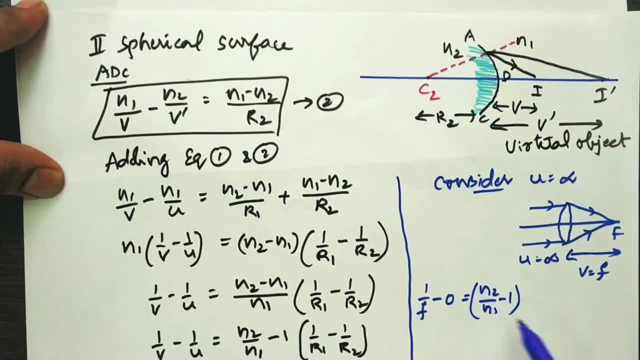 to N2 minus N1 minus 1 into 1 by R1 minus 1 by R2.. So final equation, The lens makers formula Is N2 by N1 minus 1.. Right Is N2 by N1 minus 1 by R1 minus 1 by R2.. 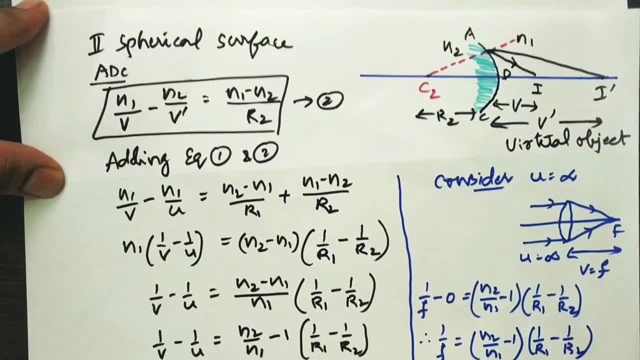 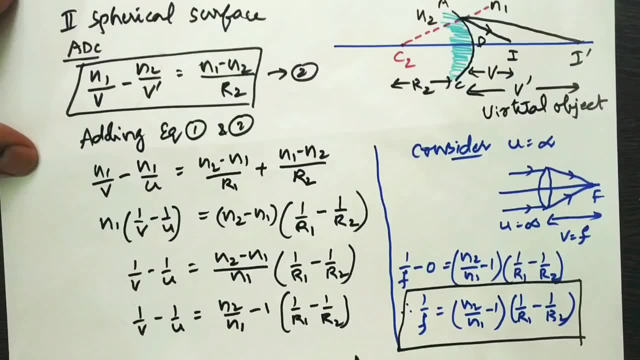 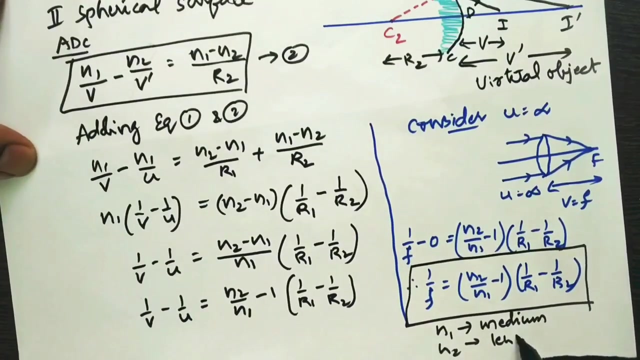 The important thing to be noted here is what is N1 and what is N2.. So please don't get confused among these two values. N1 is the refractive index of the surrounding medium And N2 is the refractive index of the lens. 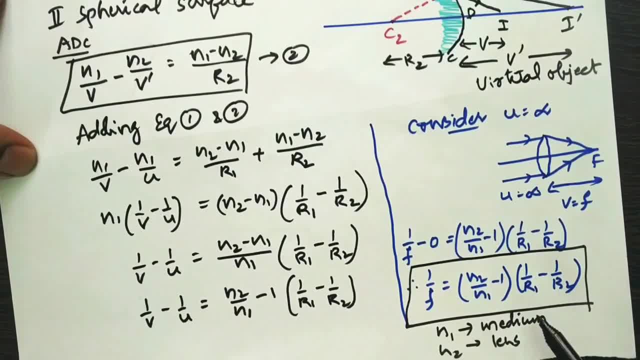 In some textbooks in the place of N1 and 2 mu 1- mu 2 also there. And in some textbooks in the place of N1 and 2 mu 1- mu 2 also there. And in some textbooks in the place of N1 and 2 mu 1- mu 2 also there. 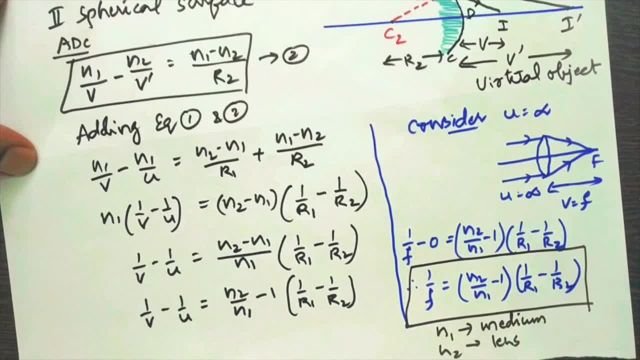 So it doesn't matter. There are 12 variables. You may follow mu 1 or mu 2, or N1 or N2.. So it doesn't matter. There are 12 variables. You may follow mu 1 or mu 2, or N1 or N2.. 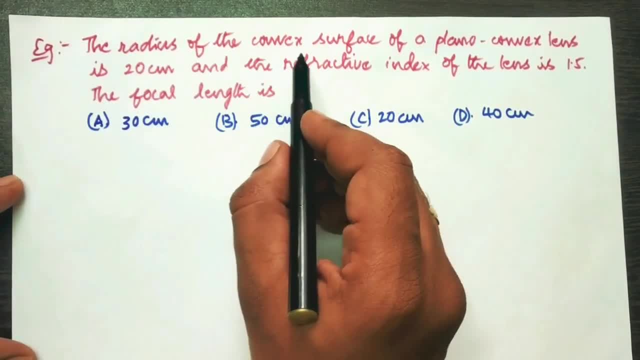 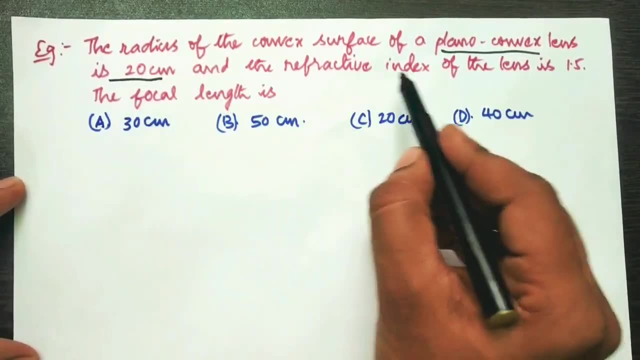 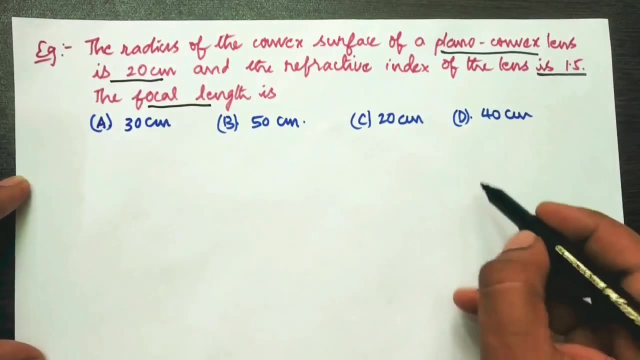 Now let us take an example problem. The radius of convex surface of a plano convex lens is 20 centimeters. So they have given us plano convex lens and refractive index of the lens is 1.5. Then focal length is. So here the plano convex lens is given. 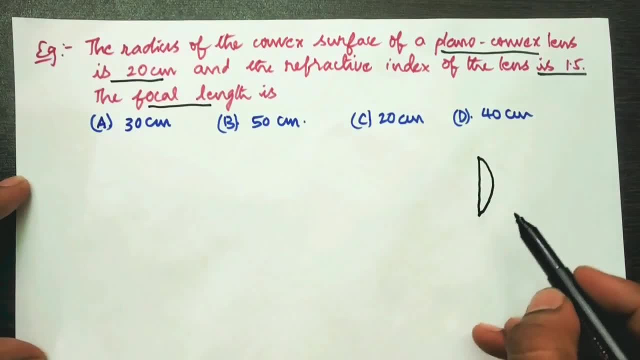 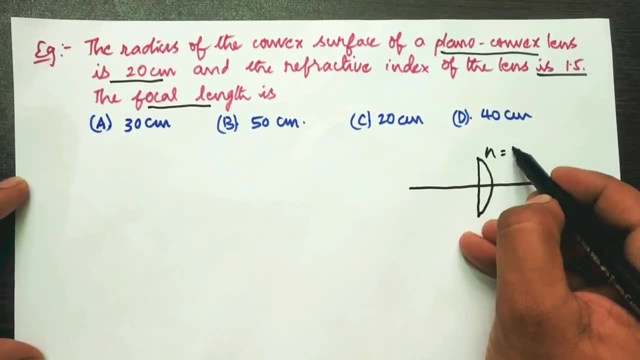 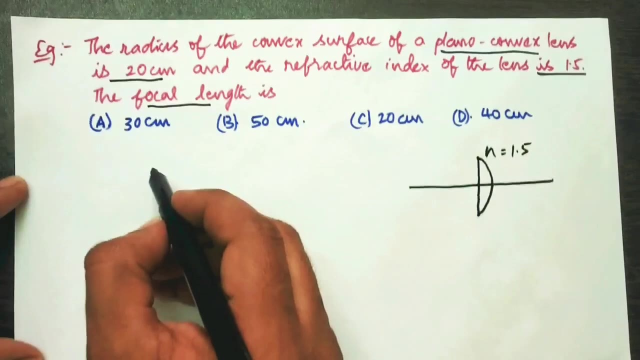 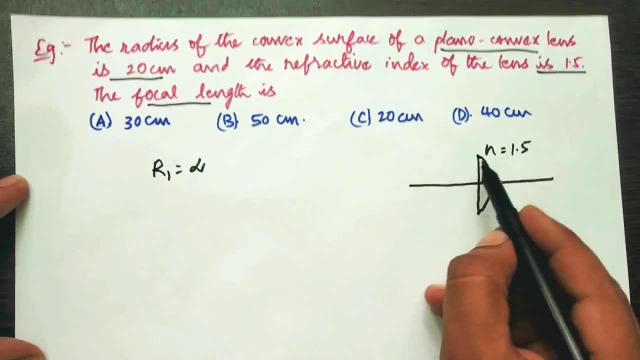 Let me draw four surfaces: Plain. And second surface is convex, Right. So let me draw the principal axis here. So we have been given the refractive index as 1.5. And the radius of curvature of the first surface. So as the first surface is plain, radius of curvature is infinity. 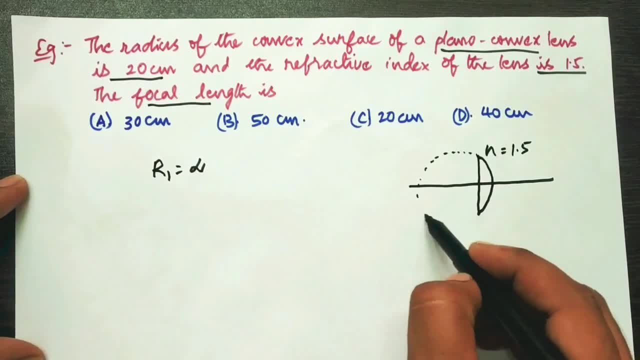 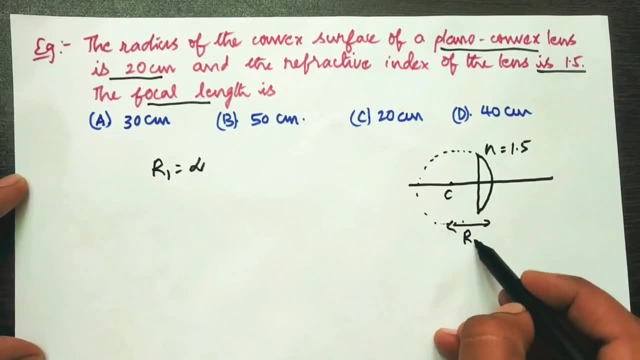 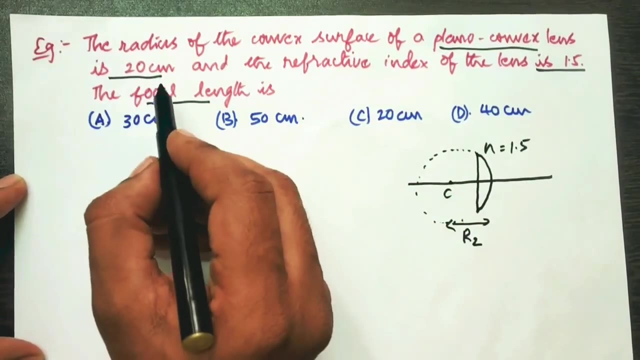 Now, second surface is something comes like this: The curved surface of second surface Right. So this is center of curvature. From here to here is called radius of curvature, So this radius of curvature R2.. They have given us the convex surface radius of curvature as 20 centimeters. 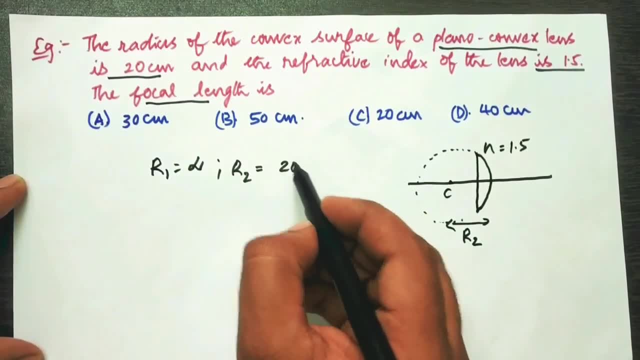 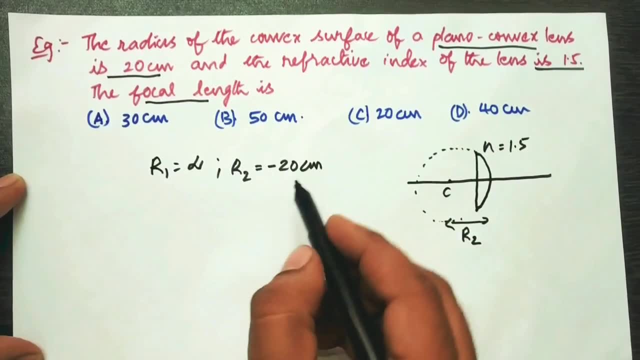 So R2 value 20.. But important thing is that the sign convention See, it is on the left side, Rather say opposite to the side of the incident race, So minus 20.. Very important to write sign conventions Now. refractive index 1.5.. 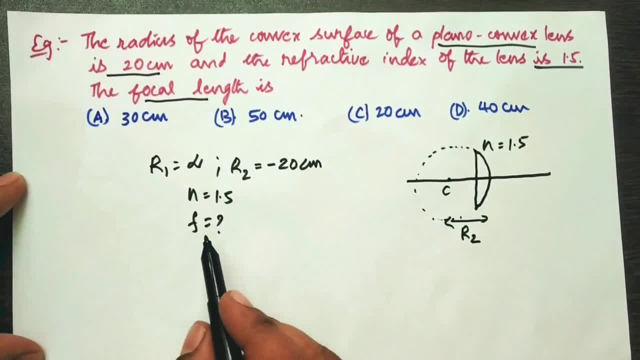 We need to find out focal length Right. So it is very clear. We use lens makers formula for finding out the focal length. 1 by F is equal to N2, N1 minus 1.. Into: 1 by R1 minus 1 by R2.. 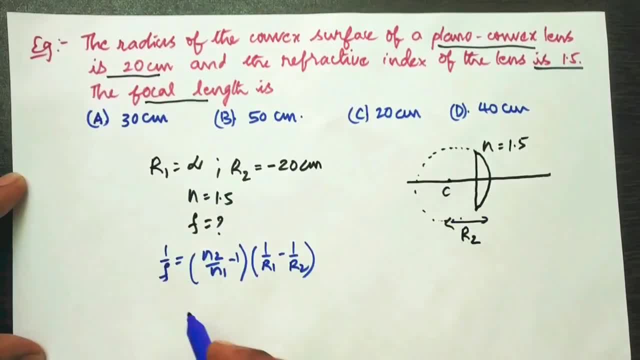 This is the actual formula, But when the surrounding medium is air, You need not write N1 and N2.. See: surrounding medium is air, So N1 is 1.. So you may reduce the formula as N minus 1 into 1 by R1 minus 1 by R2.. 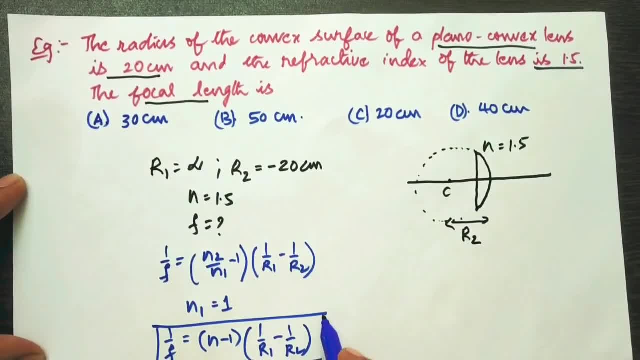 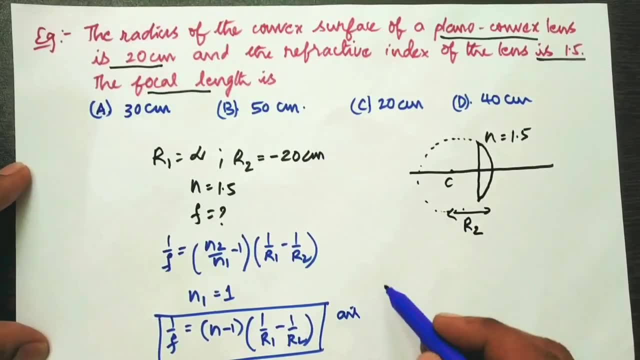 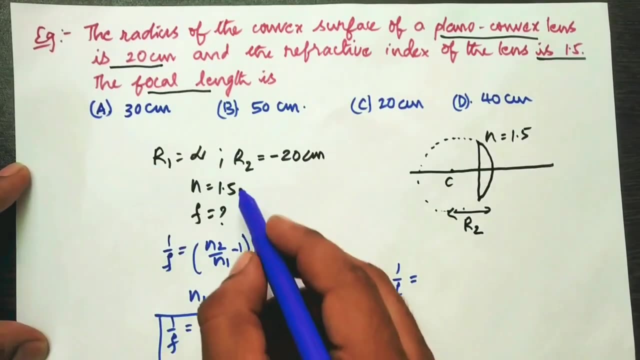 So you need not write N2 by N1.. Directly we will go with this formula: When the surrounding medium is air, Right Now we will substitute all the values here. 1 by F is equal to N minus 1.. So what is refractive index? 1.5 minus 1.. 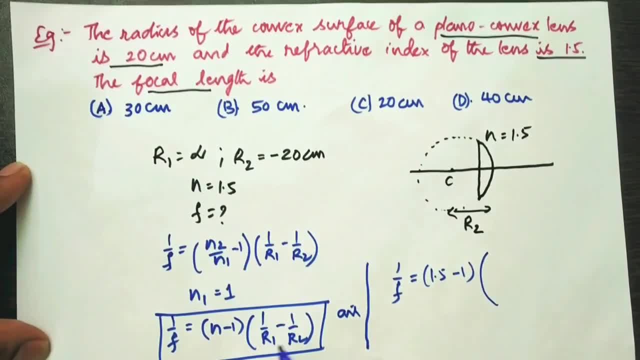 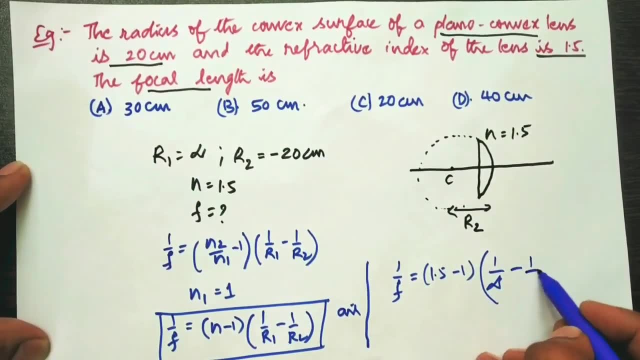 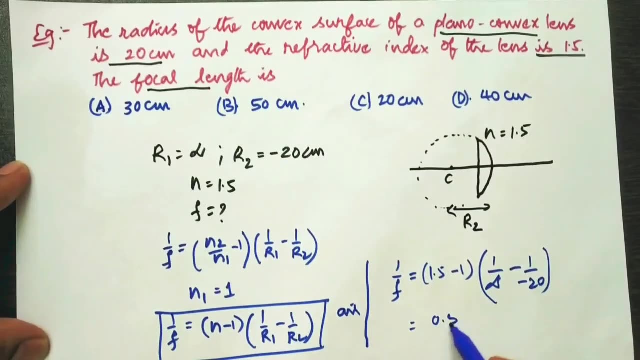 1 by R1.. The first surface is plain, So 1 by infinity, And second surface is convex: 1 by infinity, minus 1 by minus 20.. Because R2 is minus 20.. Now 1.5 minus 1 is 0.5.. 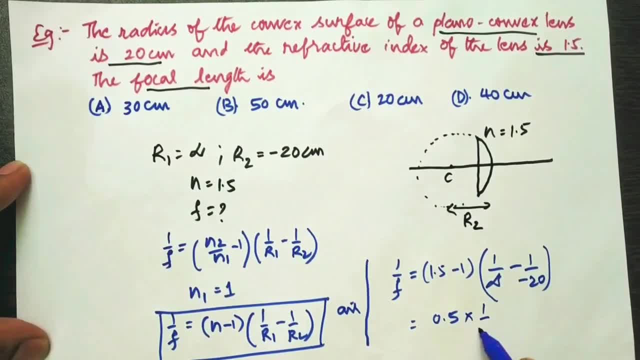 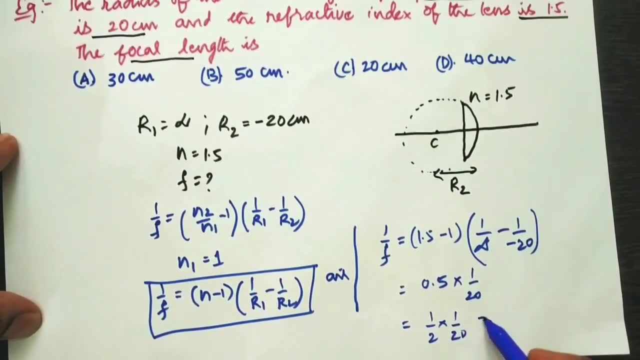 1 by infinity is 0 minus into minus plus. So I am writing directly: 1 by 20.. 0.5 means 1 by 2.. Into 1 by 20. Comes out to be 1 by 40.. 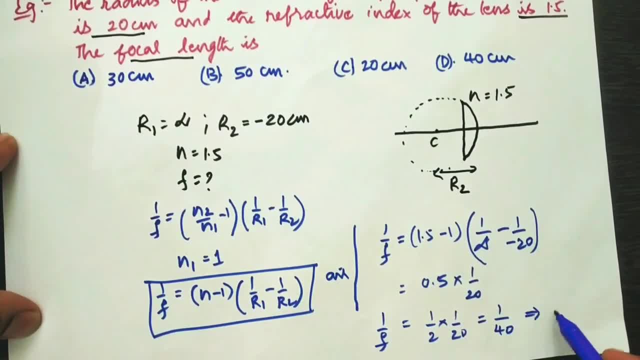 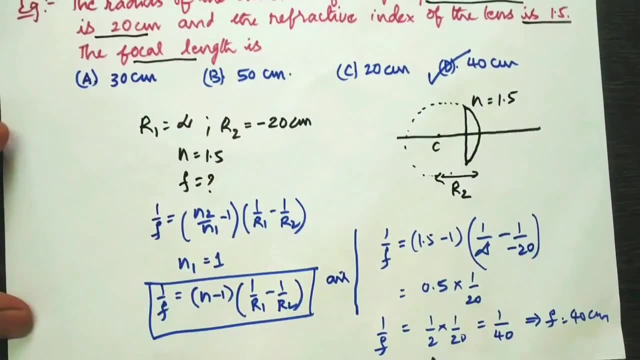 So if 1 by F is equal to 1 by 40. What is F value, 40 centimeters, Right? So the answer is option D. Like this, it is very easy for us to find out focal length of the given lens. Thank you so much for watching.